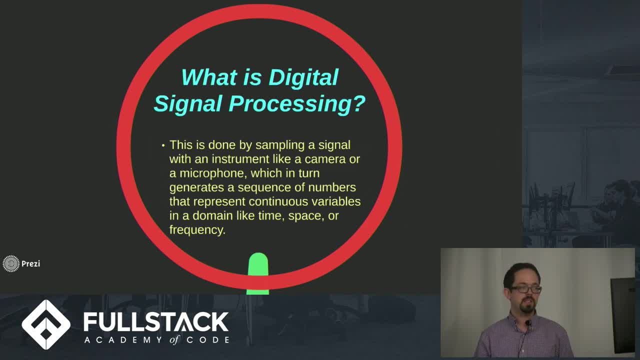 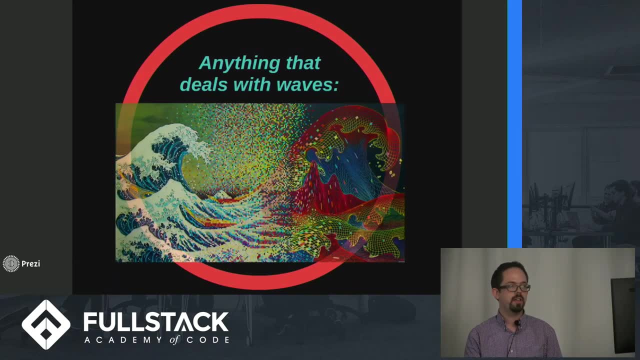 continuous variables in a domain like time, space or frequency. So what could this possibly be used for? Well, really, it's anything that deals with waves, And I love this artist's rendition of the great wave off Kanagawa. It kind of provides a great 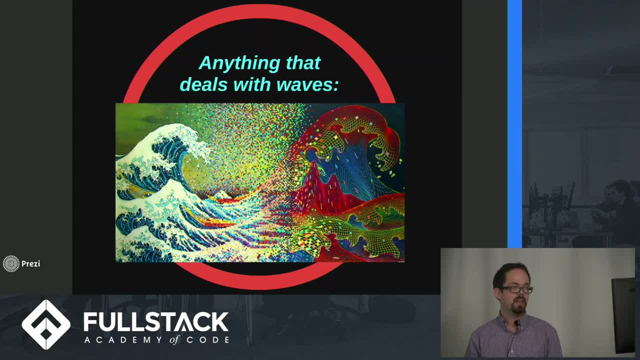 visual metaphor for it. It's a great visual metaphor for the great wave off Kanagawa. As we're talking about digital signal processing, you have the natural waveform on the left being mapped and translated into the digital graphical representation on the right. So if we're dealing 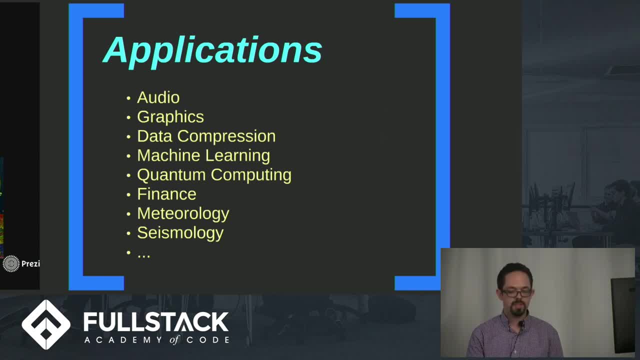 with audio, that means we're talking about sound waves. Graphics or images are light waves. As you can see, the list really goes on and on and on For any kind of data that's going to repeat over time. there is one application which is not recommended for digital signal processing. 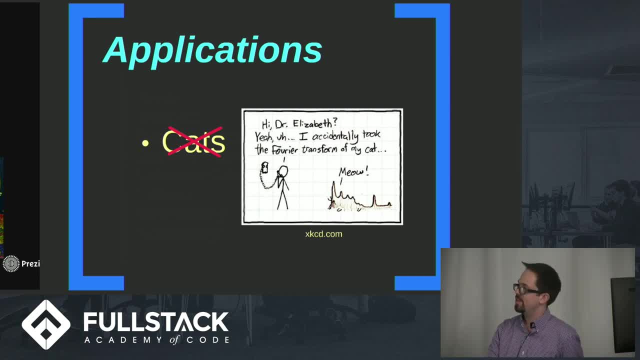 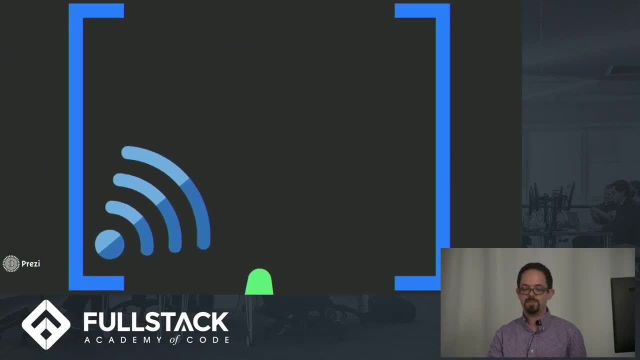 That would be Katz. Katz does not appear to be happy to have his fast Fourier transform taken. So we can get various types of signals through sampling. but once we have that information, how can we translate it into data that we're going to analyze, change or recreate? 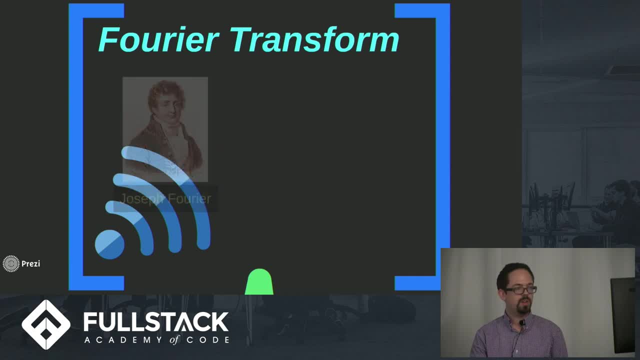 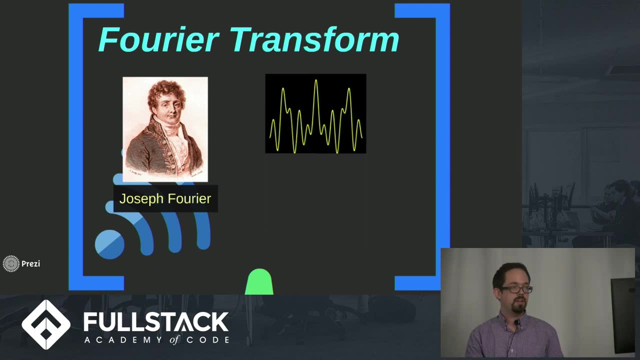 That's where the Fourier transform comes in. There was a French mathematician named Joseph Fourier who had this crazy idea that a complex waveform- it could be light, heat or sound- can be essentially broken down into its component parts, which is just a group of simple sine waves. 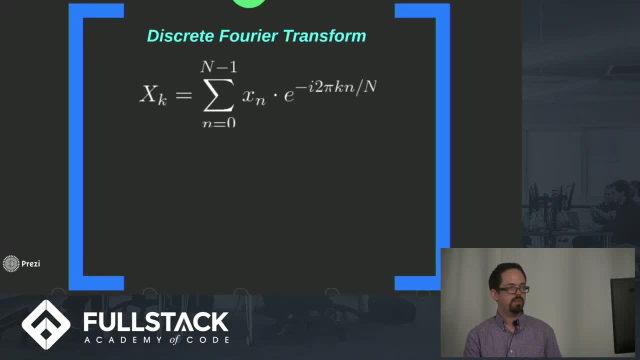 And this is the equation that he came up with to do that. It's called the discrete Fourier transform. Essentially, the discrete Fourier transform is a mapping of data between two domains. We take input in the time domain and we get output in the frequency domain. We use zero-based indexing. 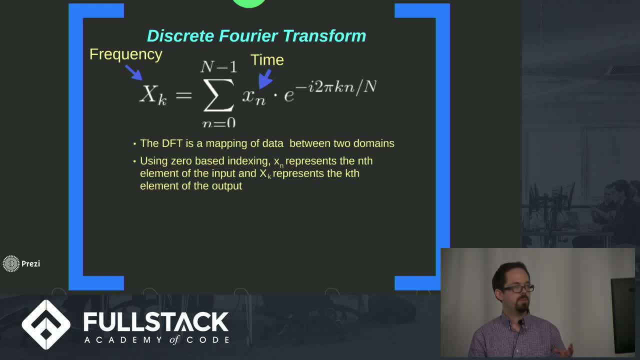 where you can see lowercase ns. It starts at zero and we're summing up until n minus one. X sub n represents the nth element of the input and x sub k represents the kth element of the output. Lowercase x denotes our time. 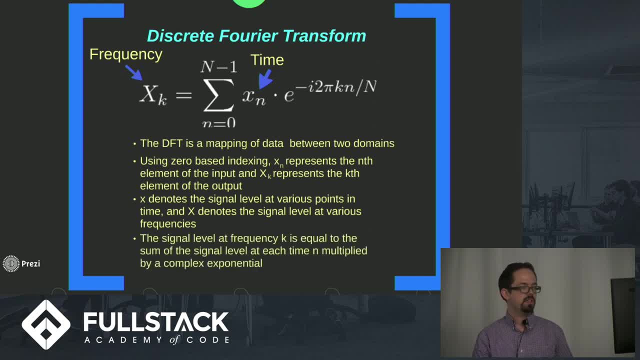 signal. uppercase x is our frequency signal, and the signal level at frequency k is just equal to the sum of the signal level at each time, n, multiplied by that complex exponential that you see on the right. Wow, that's a lot of math. So what I'm going to do next is make an analogy to kind of talk about. 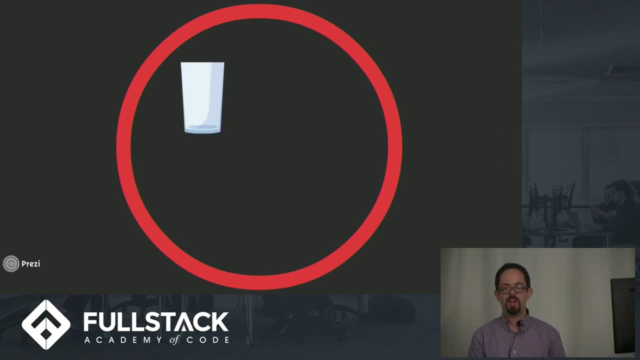 what really is going on here. So let's say, I went down the street to the juice bar and I got this delicious apple-carrot juice and I liked it so much that I wanted to be able to make it again at home. So let's say, in theory, I could take the Fourier transform of this juice. Well, what that? 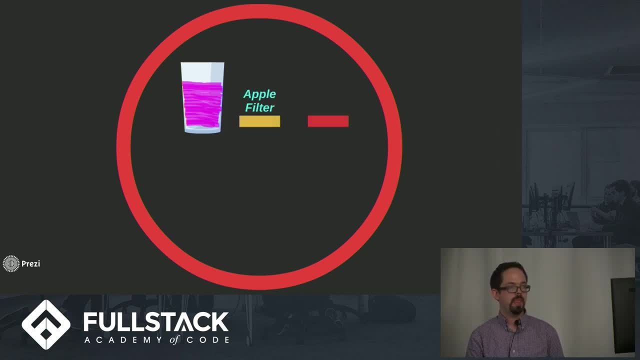 would mean is setting up a couple filters. We could have an apple filter and a carrot filter, And if we pour this juice through the various filters, it's going to return the number of apples, say, one apple and the number of carrots. So now I've gone from juice to the 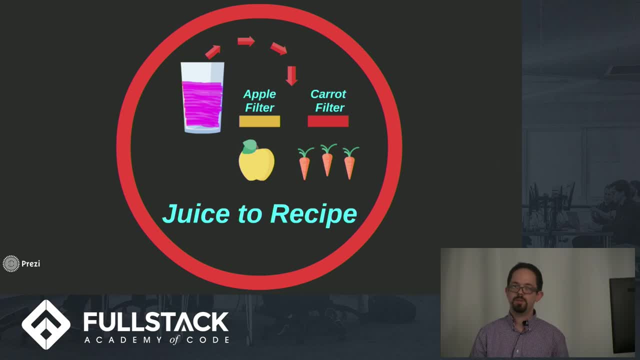 recipe, And if I wanted to make this again or improve upon the recipe, I could do that, And so, essentially, that's what the Fourier transform does. The Fourier transform takes a waveform and finds its recipe. So now that we know a little bit about how this algorithm works, let's take it. 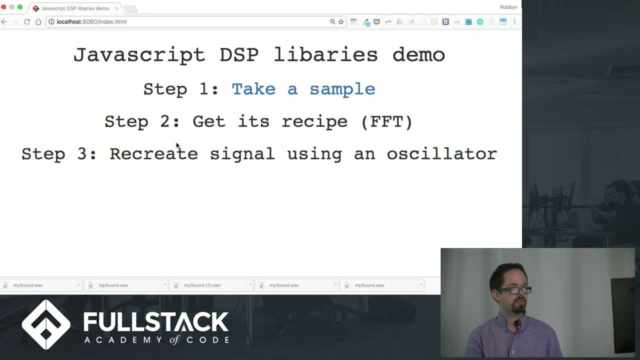 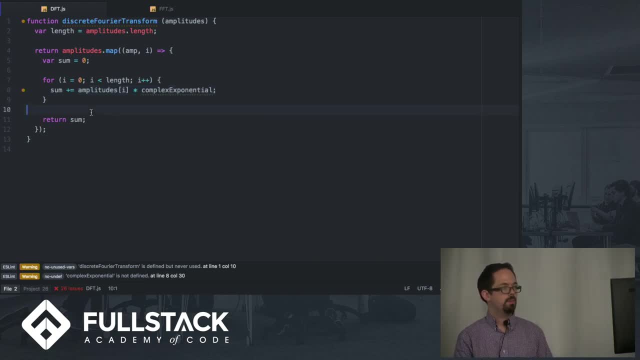 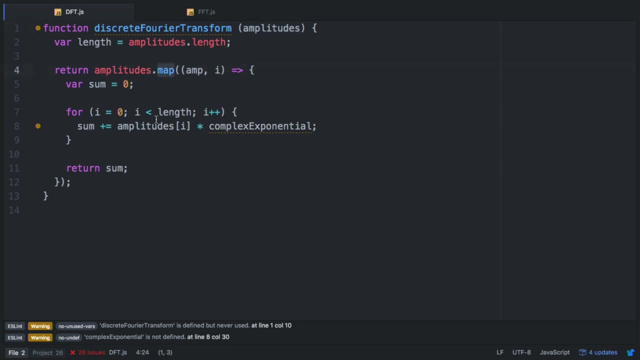 take a look at what it might be to implement this in JavaScript, And I have here just a really basic implementation. It's not actual code, It's really pseudocode. But you can see, our Fourier transform function is going to take some amplitudes. These are complex numbers And it's going to map over these amplitudes. We're going 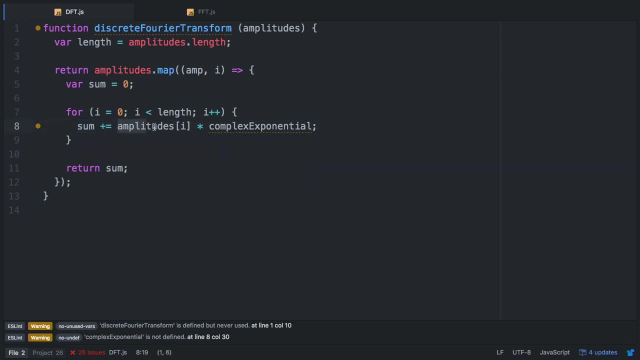 to set up a sum And at each point in the amplitudes, we're multiplying the amplitudes by the complex exponential which is creating this sum, which is returned back to the amplitudes array. Now, as you can see, this algorithm would really take a long time to run Its computational time. 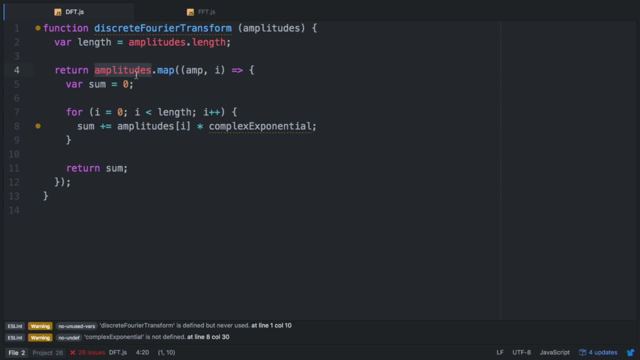 would be O of n squared, because we're essentially multiplying the sample size times itself. That's why, in the 1960s, there were two researchers, James Cooley and John Tuckey, who wanted to improve upon this, And they came up with what is known. 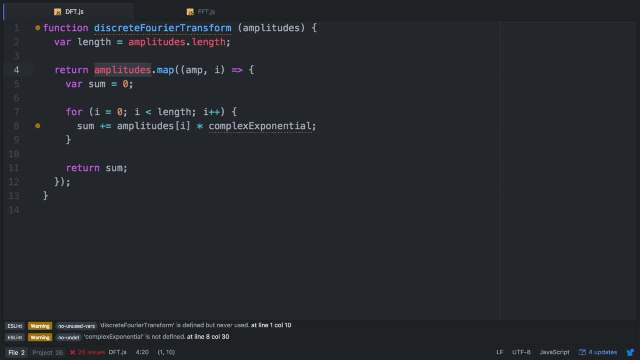 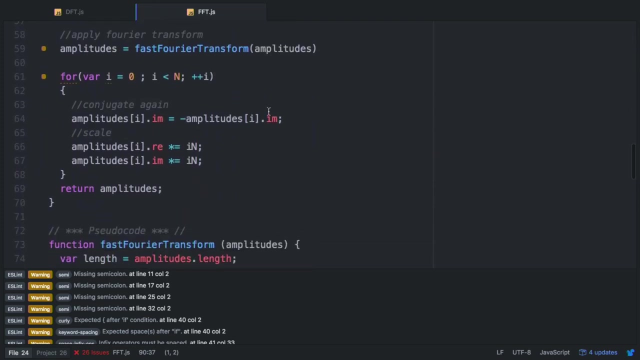 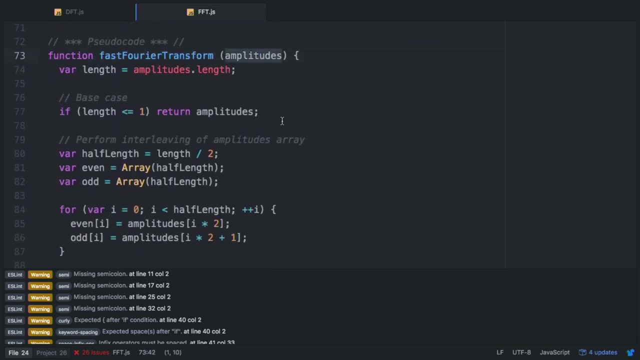 as the fast Fourier transform. They were able to re-express this discrete Fourier transform recursively to reduce the computational time to O of n log n, which is a lot faster. And here's our example. sorry, fast Fourier transform. Okay, And so again it's simply taking in this array of amplitudes. 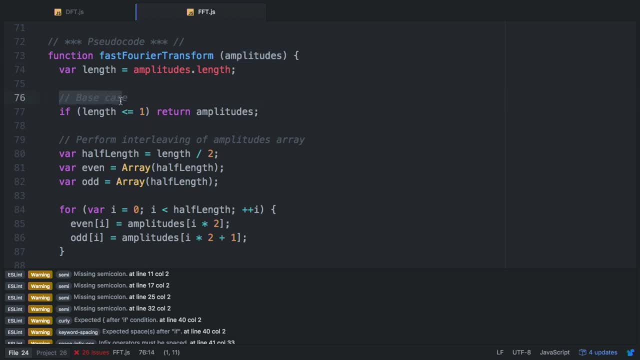 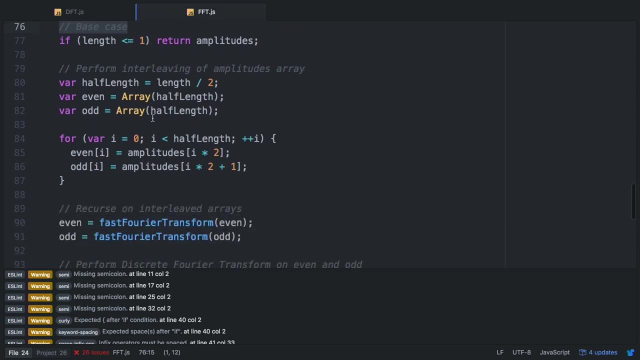 Since it's a recursive algorithm, we have to set up a base case where the length of the amplitudes array is less than or equal to one. We're simply going to return that array And the algorithm basically applies a divide and conquer strategy where it takes the amplitudes. 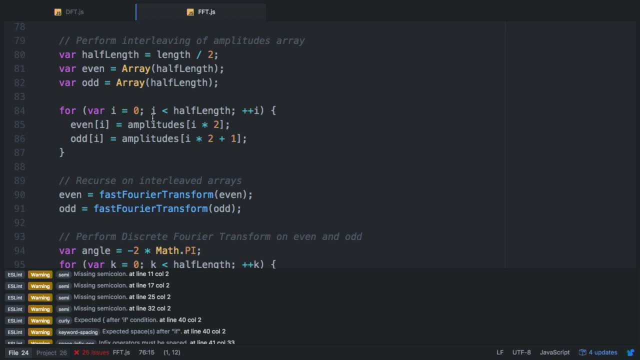 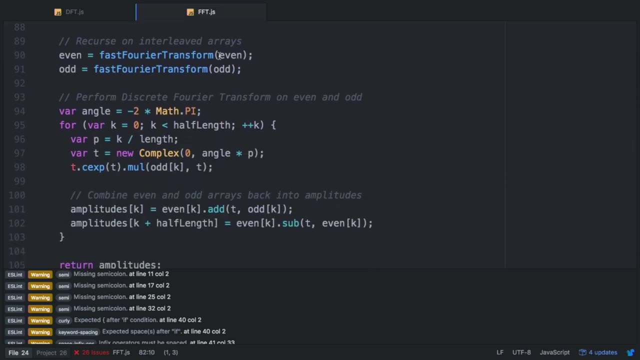 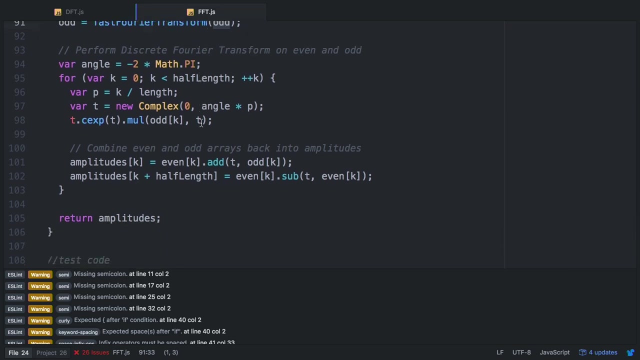 array performs an interleaving, breaking it up into an array of the even indexes and odd indexes, Then it recurses on each of those interleaved arrays and performs the discrete Fourier transform, And then it does the discrete Fourier transform on the smaller arrays. as these recursive cases return. 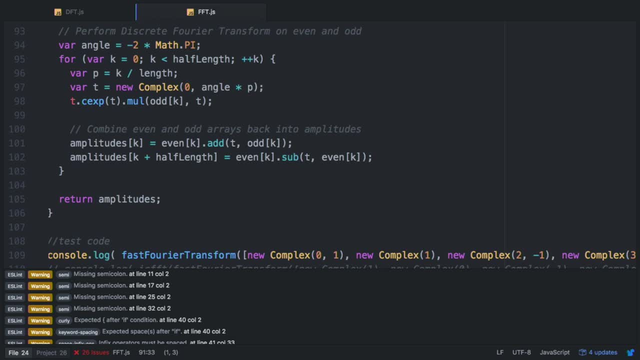 and then combines them at the end. Now, obviously, I'm giving you a really fast overview of this fast algorithm, which doesn't get into the complex math that's involved in combining the arrays, And that's because to do that would really require a math lesson or two in and of itself. 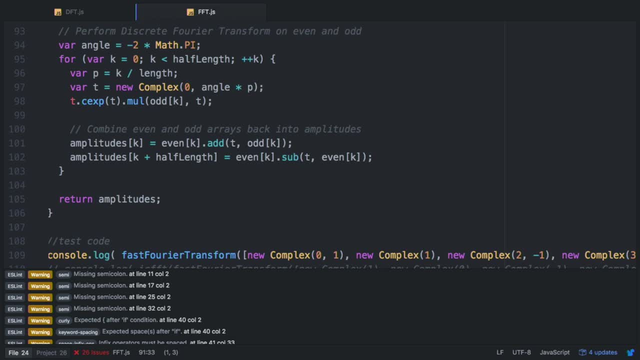 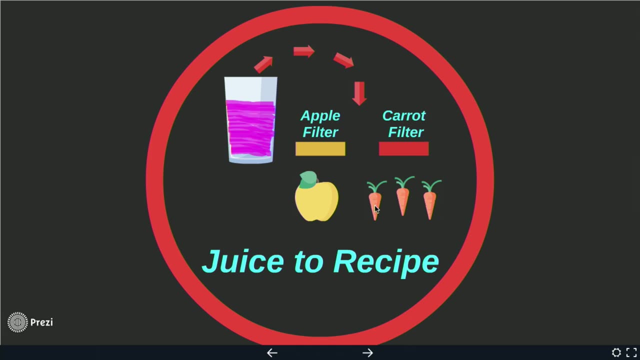 which I don't have time for today. And this sort of brings me to another great point that I have is that, as developers, we don't have to implement these algorithms in our programming language of choice, because there's many great libraries which are going to do this for us, And there's 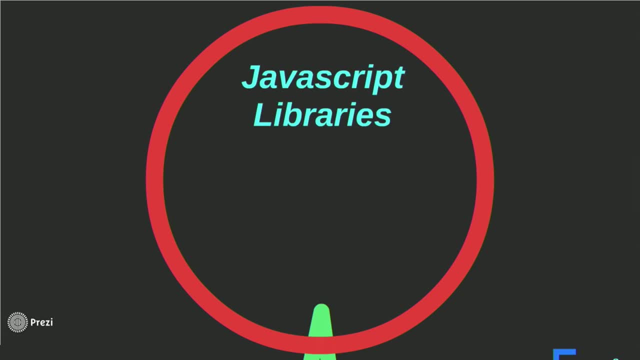 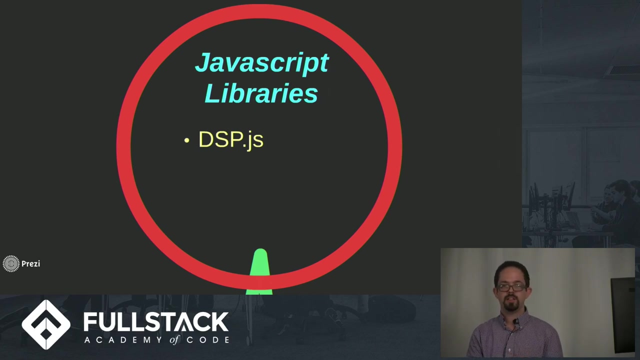 a few JavaScript libraries that I want to talk about which we can leverage to get Fourier transforms of some kind of data that we're working with. There's DSPJS, which I like because it implements an FFT object and really kind of gives you access to the inner working. 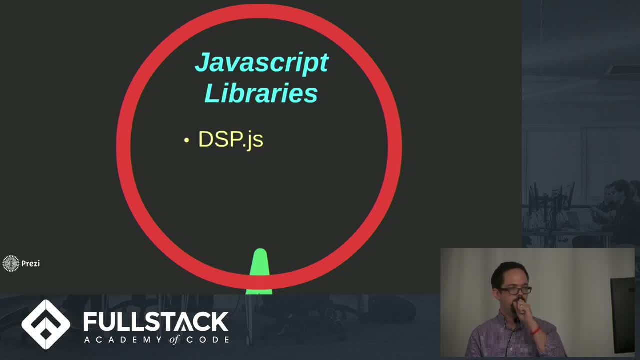 of how an FFT would function. There's also p5.js, which is really cool because it's sort of geared towards artists who want to visualize data. It could be sound data or any other kind of waveform that you want to visualize, And also the Web Audio API is able to take the fast Fourier transform. 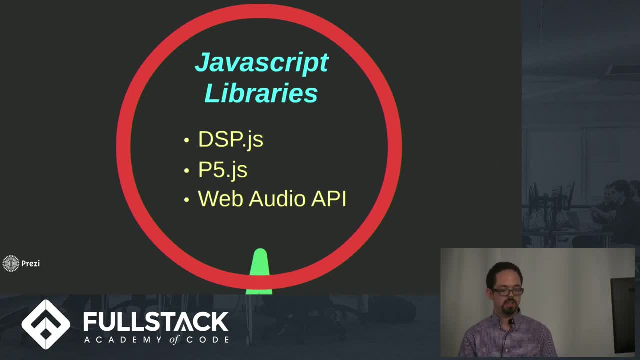 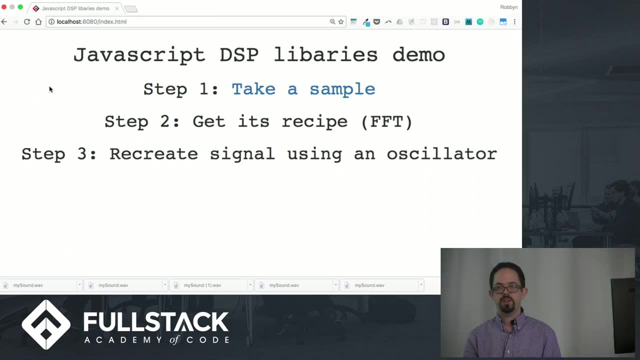 of audio and basically give us the frequencies. So I've built a small app that I have running here to kind of show you a little bit about how these libraries work, And what it's intended to do is basically take a sample, get the recipe of that audio sample. 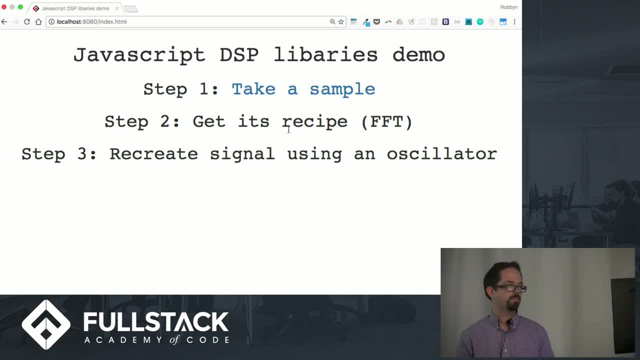 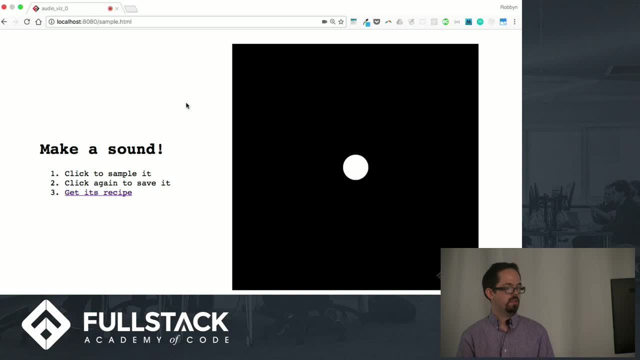 and then it's going to recreate the signal using an oscillator. So let's get started. This is a really cool little sound recorder that I found. I'm going to take a sample of myself whistling here Now. if I click again, it's going to save that and play it back for me. 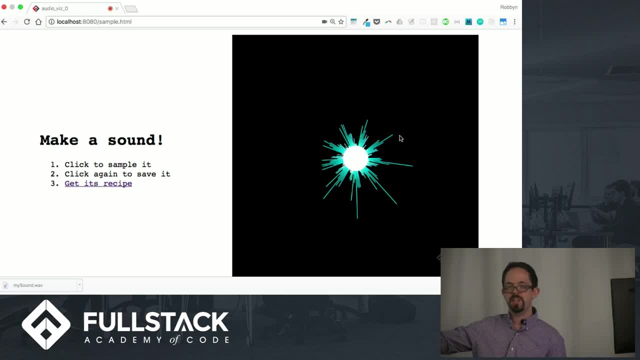 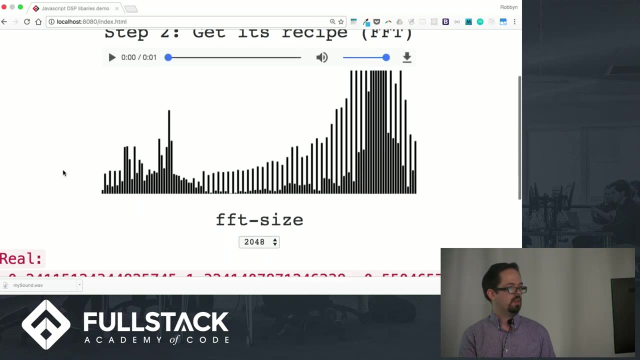 And we saw a really neat visual representation of the frequency data that the p5 FFT is returning. We're just mapping that to these different rectangles around a circle here. So now let's go back and see what the recipe of this audio data would be. Here is sort of another fun canvas, which 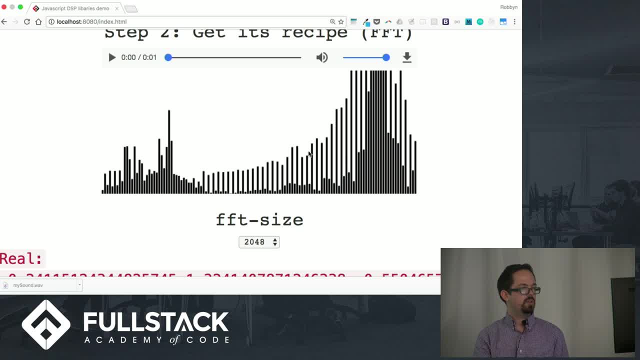 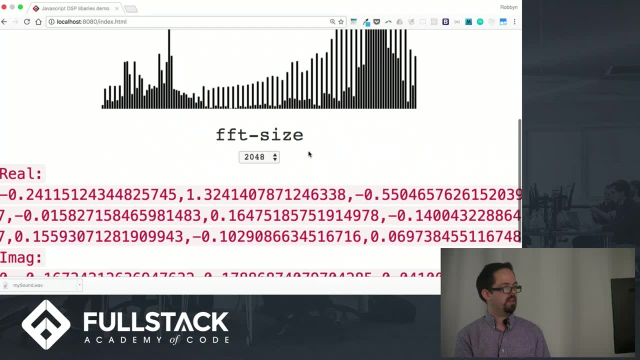 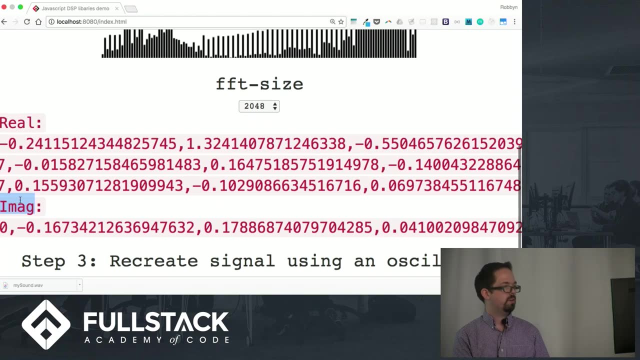 is mapping over our FFT and returning the frequency levels at different points in our sample Below that I wanted to show. these are the two arrays that the FFT is going to return. We have points in the real space and imaginary space which kind of, if you remember, vectors. 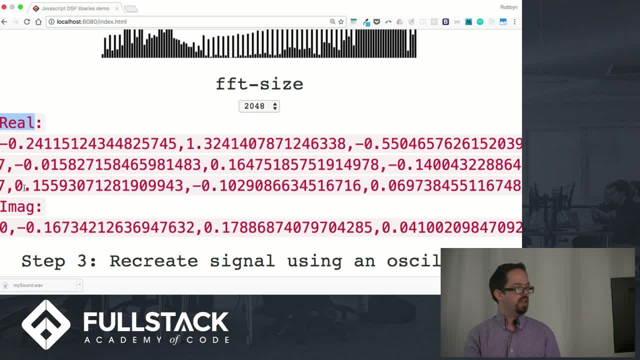 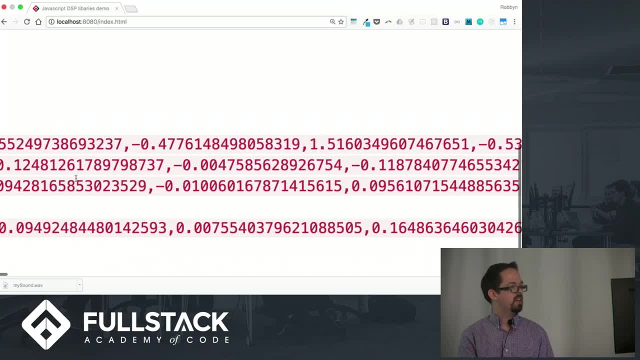 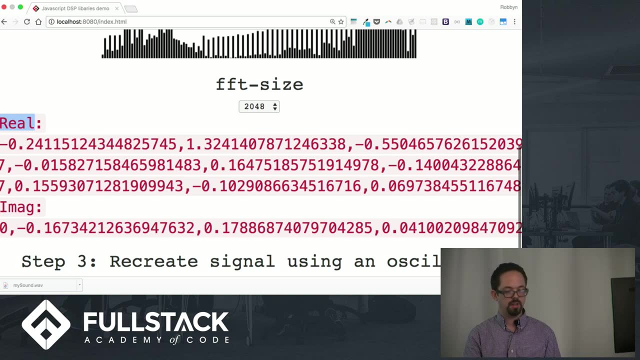 like. that's how we compute a vector on a graph And together those are the complex numbers that we're returning. As you can see, these arrays kind of go on and on and on, because we're sampling 2048 different samples of that audio signal. 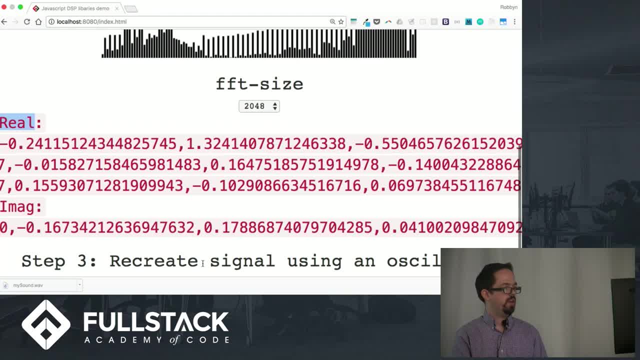 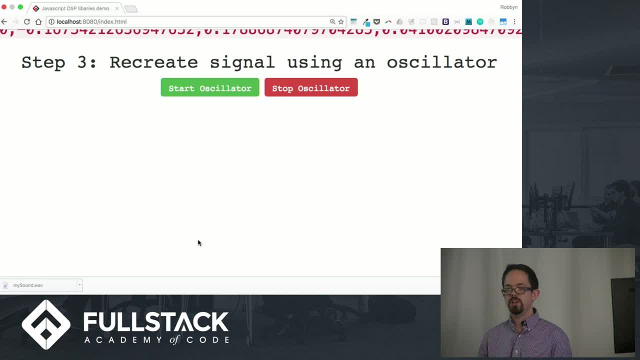 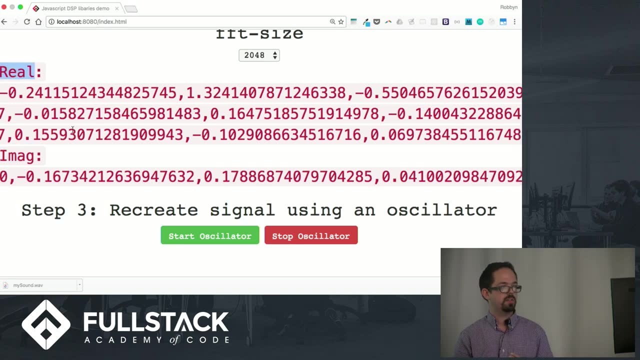 And finally, what we want to try and do is recreate that signal. And the Web Audio API has this really great thing where you can set up an oscillator and then you can create a periodic waveform with that oscillator. And what I can actually do is take these FFT arrays, the real and imaginary arrays, pass it to that oscillator. 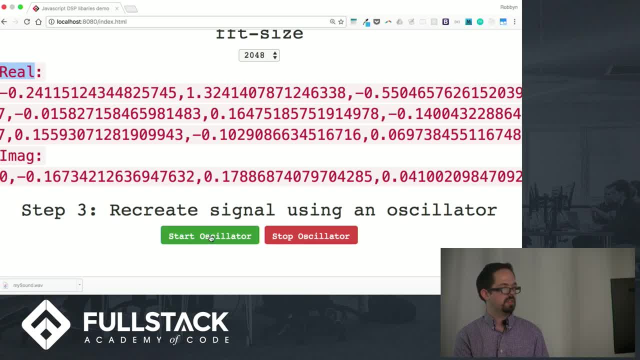 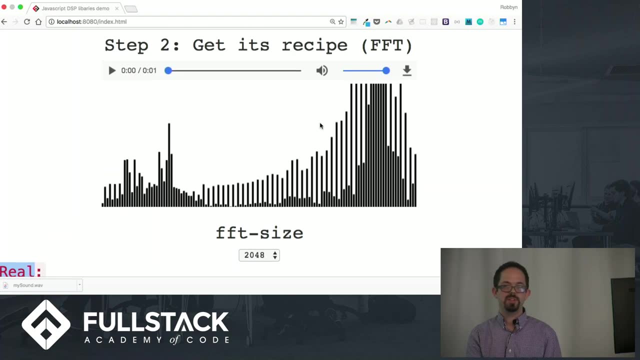 and it's going to oscillate at these frequencies. So let's hear what that sounds like. Cool. So not quite exactly how my whistle sounded. It's a little bit fuzzy and kind of rough around the edges, And one of the reasons for that is probably the FFT size that we're taking The Fast. 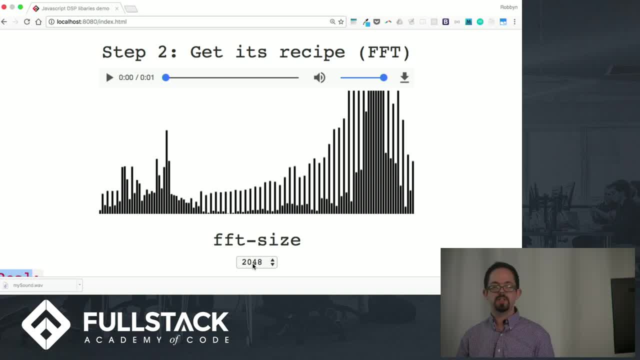 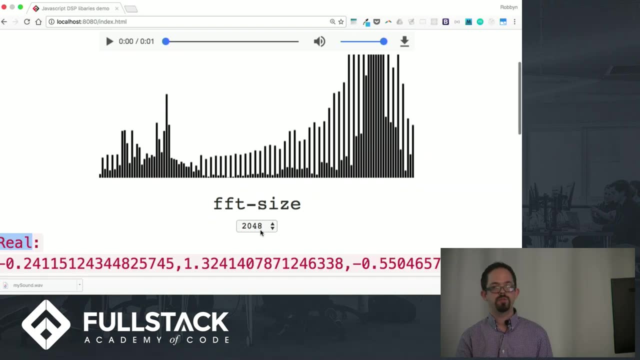 Fourier Transform can come in many different sizes. The particular implementation here is what's known as a Radix II implementation of the Fast Fourier Transform or Base II, where basically the FFT size has to be a multiple of two because it's performing that interleaving.